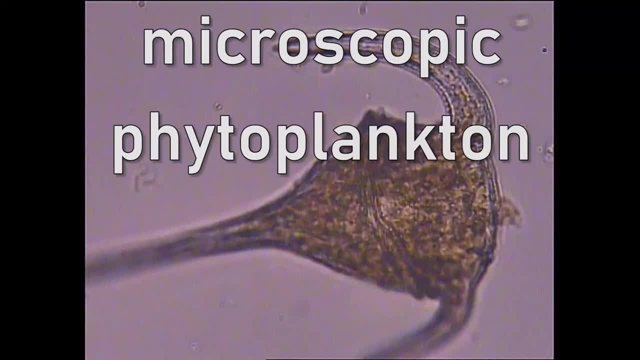 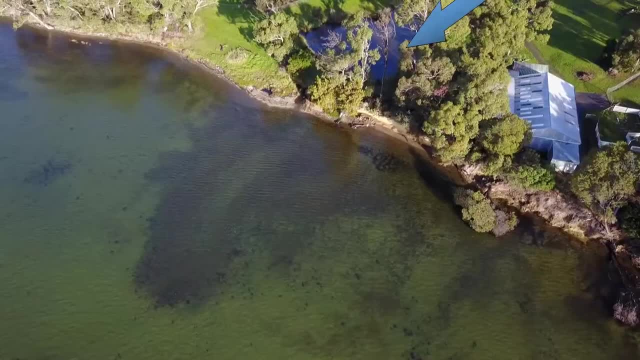 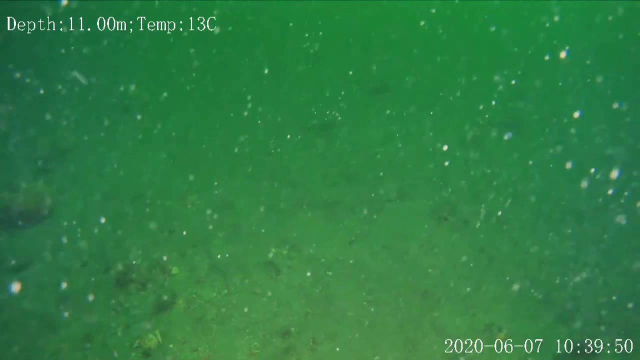 around, so seaweed and phytoplankton can directly absorb these nutrients from the water. The source of these nutrients for plants in the sea can come from a number of places. Rainfall onto land can wash nutrients out of the ground into streams and rivers that end up in the sea. At sea bacteria 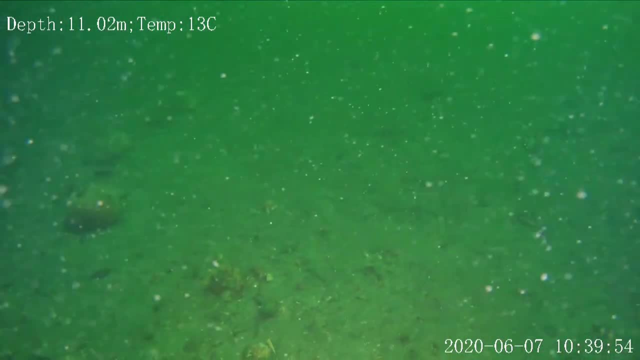 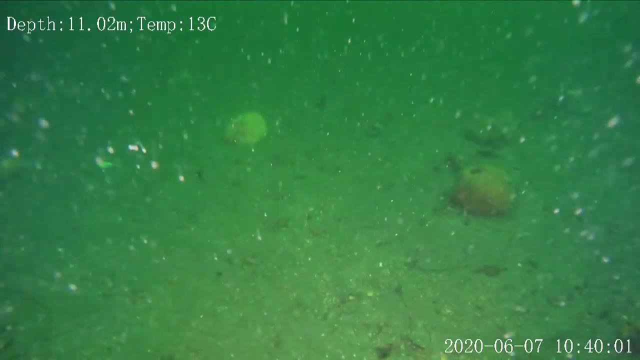 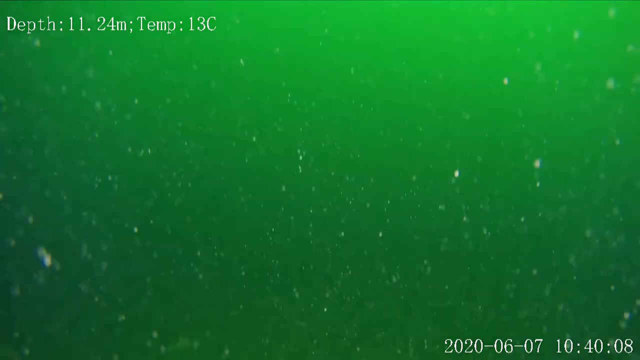 will eat or consume the remains of dead organisms. This biological debris floating around, made up of organic matter from dead seaweed, plankton and animals, sinks to the bottom of the sea floor as marine snow, where bacteria break them down into more simple chemical nutrients. These nutrients can be picked up by the water. 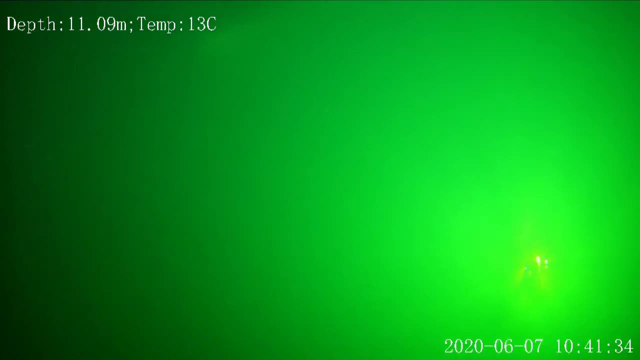 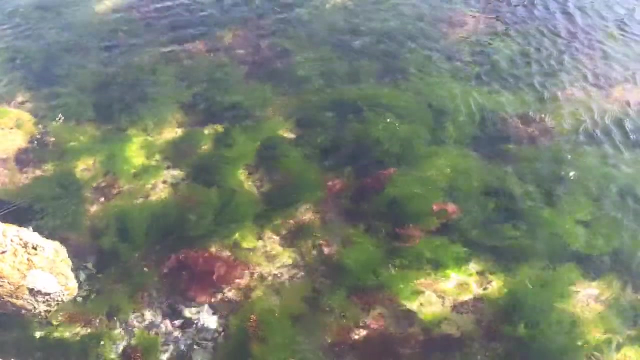 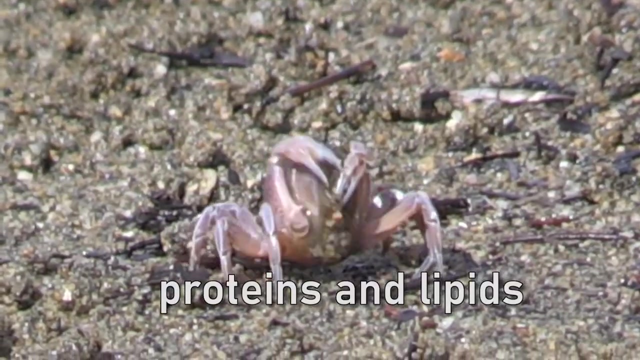 currents and returned to the sea surface to be taken up by phytoplankton and seaweed to start the cycle anew. Nutrients for seaweed and phytoplankton tend to be pretty simple chemicals, but animals need more complex nutrients to stay alive, such as proteins and lipids. 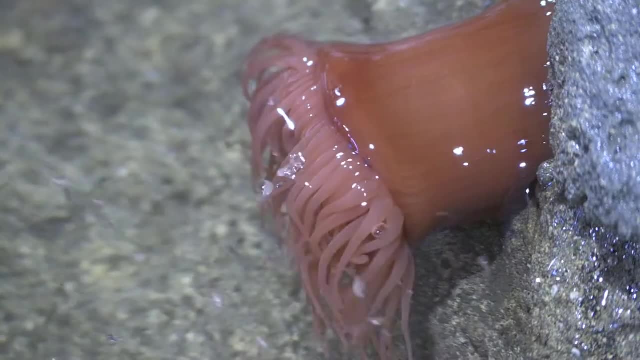 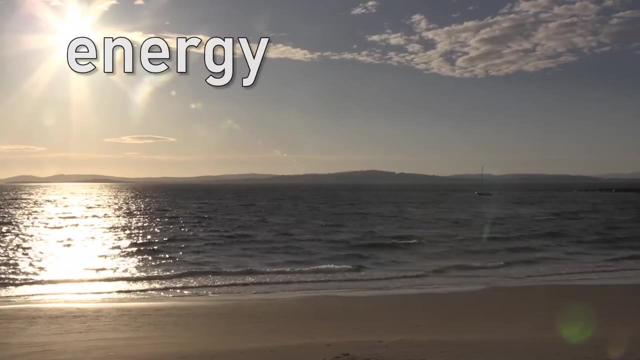 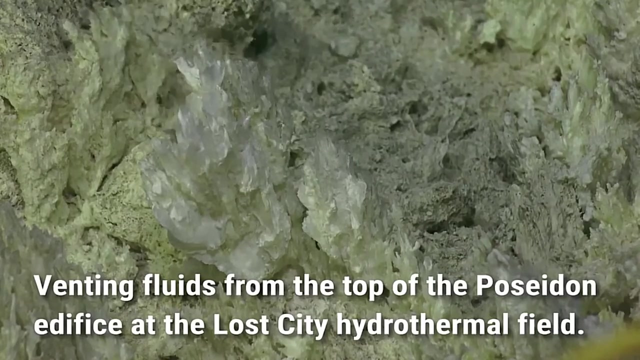 Instead, these chemicals are usually found inside other living organisms, so animals need to eat or consume these organisms to obtain the nutrients. Without a source of energy, life on planet earth would not exist. The primary source of energy for life on earth is the sun. Another source of energy, a minor one, is the heat coming from the hot rocks. 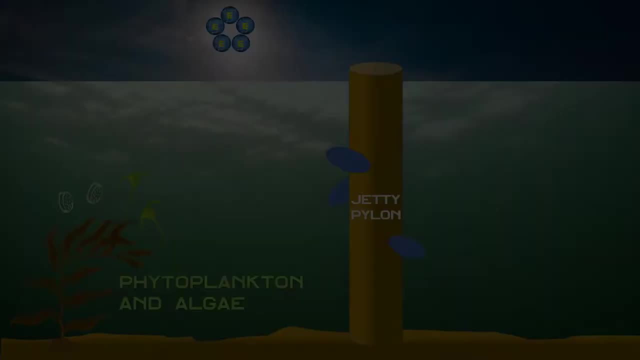 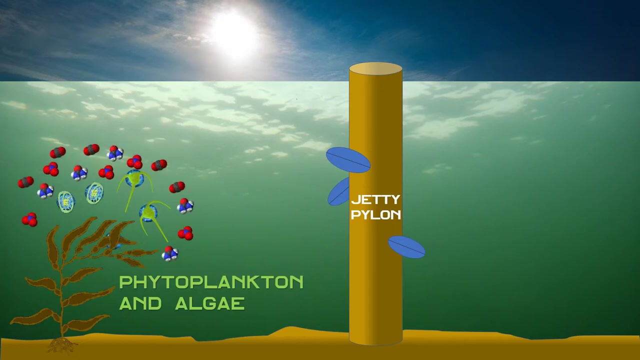 deep in the earth, but we won't be covering that source of energy in this video. Plants and algae obtain energy from the sun, Using carbon dioxide and nutrients from the environment as primary building blocks. plants are able to combine these chemicals with sunlight to produce different chemicals to help them grow and survive. 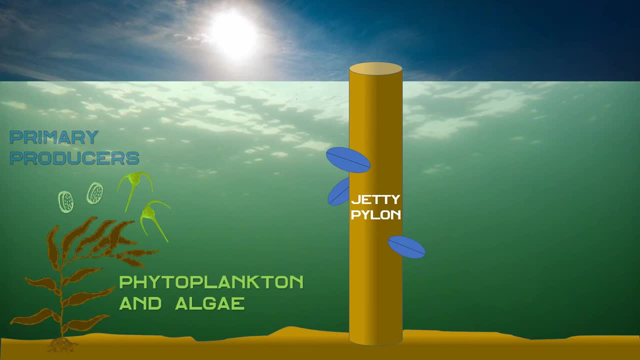 We call plants and algae primary producers. This process converts sunlight energy into chemical energy and it's called photosynthesis. Animals that obtain their chemical nutrients and energy by consuming plants are called primary consumers. Examples of primary consumers in the sea include zooplankton. 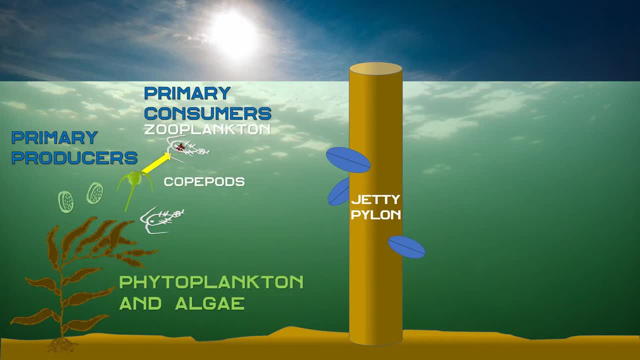 such as copepods, which eat phytoplankton. These animals have consumed and obtained the energy and nutrients from the plants and now have it as part of their body. Some of the energy and nutrients are lost by the animal through breeding or faeces or using the energy to move. The rest is now. 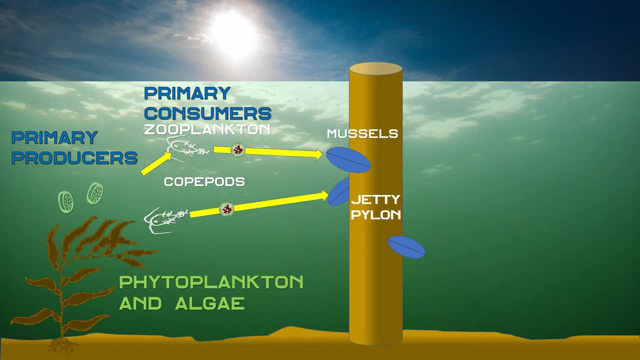 part of the animal's body, which means another animal can come along and consume them and obtain the energy and nutrients. We call these secondary consumers. Mussels are a type of secondary consumer, but they also eat phytoplankton. Now we have a chain of things eating other. 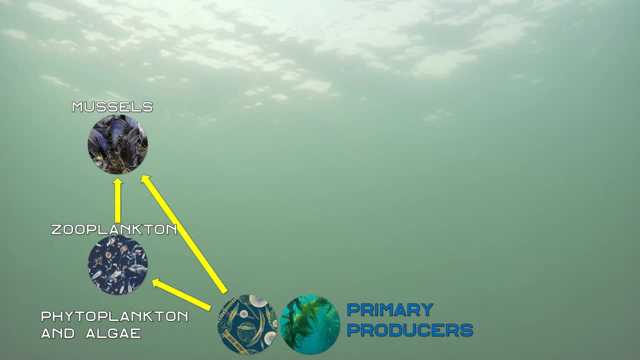 things, starting with primary producers, followed by primary consumers, followed by secondary consumers. hence the term food chain. We use arrows to show what the consumers are feeding on, and the arrows also represent the flow of energy and nutrients up the food chain. As we go up the food chain through different levels, we call these trophic levels from the 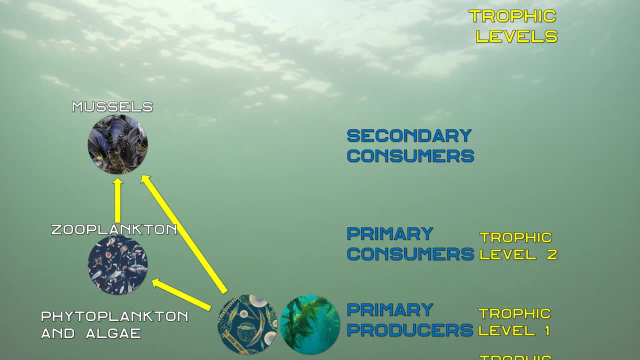 Greek meaning nourishment. The base of the food chain are primary producers at trophic level 1. As we move up each level and the consumers eat those from the levels below, there are always some bits left over, like uneaten pieces of animal and faeces released by the consumer. 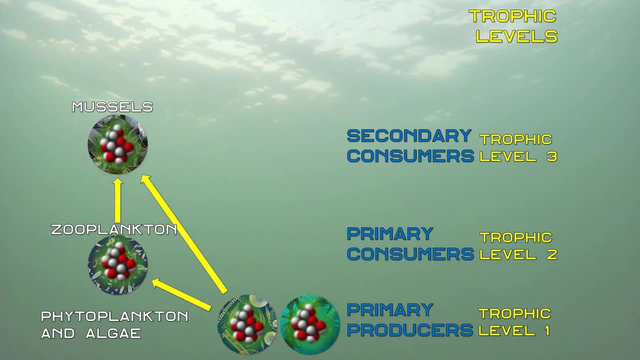 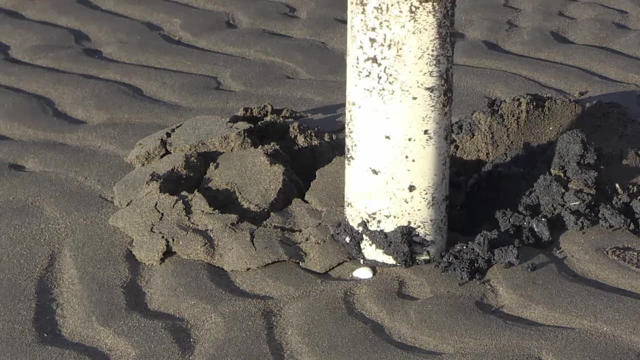 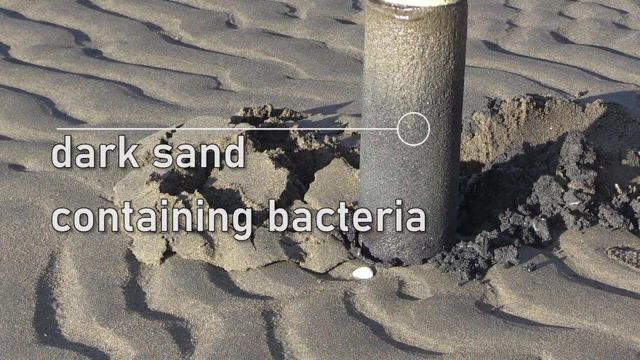 This organic matter still contains valuable nutrients and energy, so other organisms make use of this matter, and we call them decomposers. These can be microscopic, such as bacteria as indicated by the different colours of sand below a beach Decomposers- Decomposers. 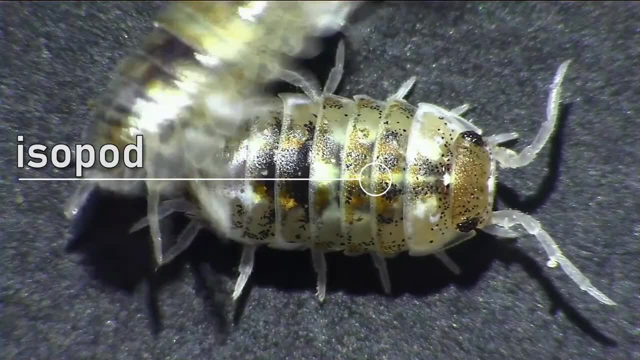 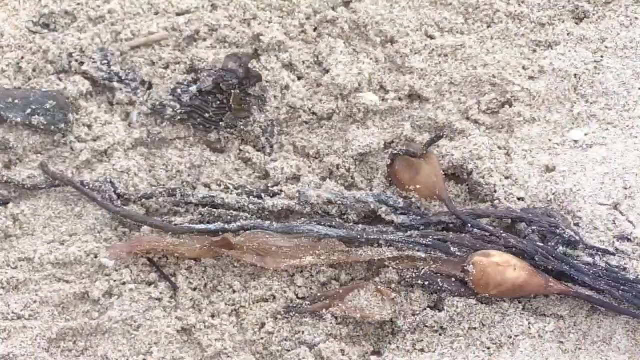 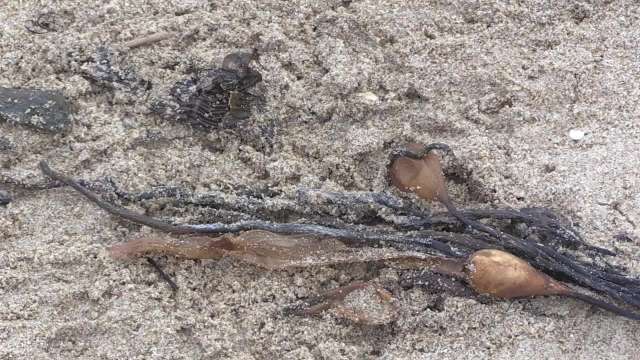 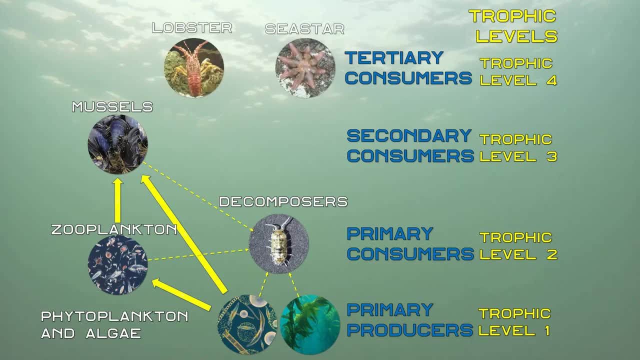 Decomposers are a vital part of the ecosystem, as they recycle nutrients which are then available for plants to use. Otherwise, the organic matter will simply become sediment at the bottom of the sea. Once we get above the trophic level 2, any consumer eating another consumer is called. 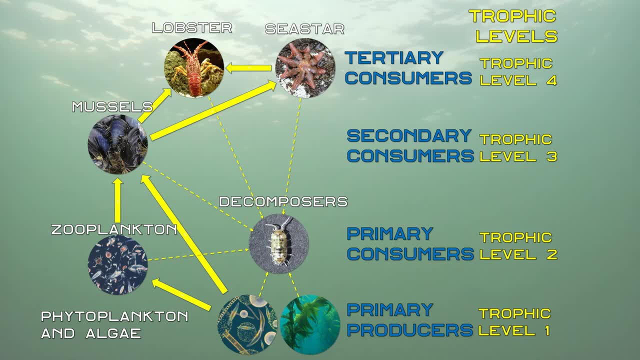 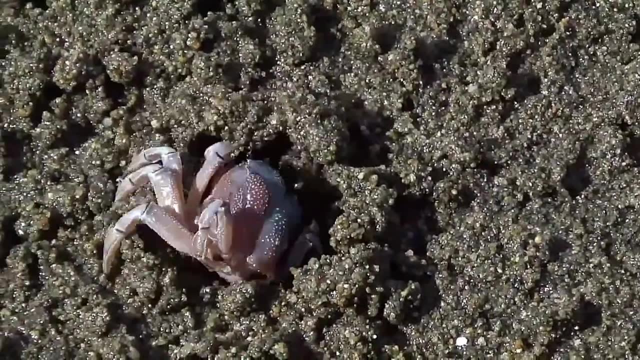 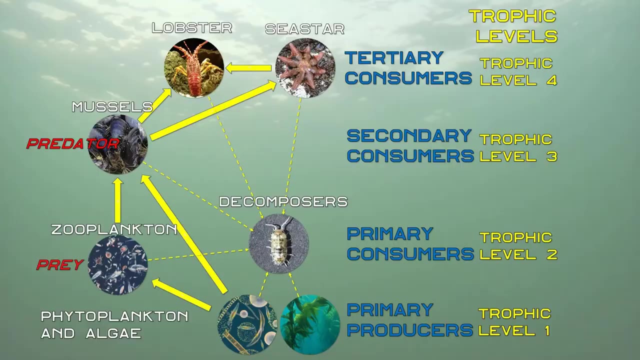 a predator, The animal that is being eaten is called prey. This creates a situation where prey species develop strategies to avoid being eaten, while predator species develop more efficient techniques for obtaining prey. Also, with more levels, the predator-prey interactions become more complex. 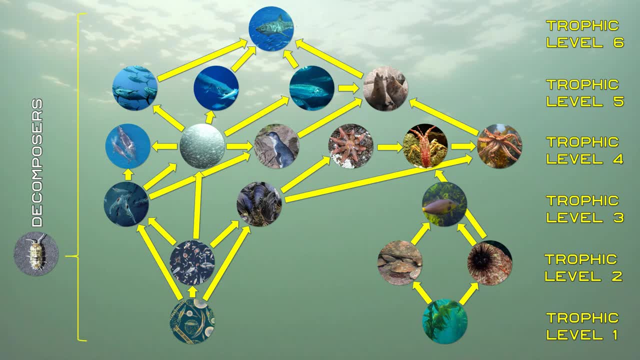 Some animals eat other animals on the same trophic level. The arrows showing the flow of nutrients and energy up the food chain start to cross each other, and what started off as a simple food chain has now become a complex food web. There are some other interesting things to note about the food web. 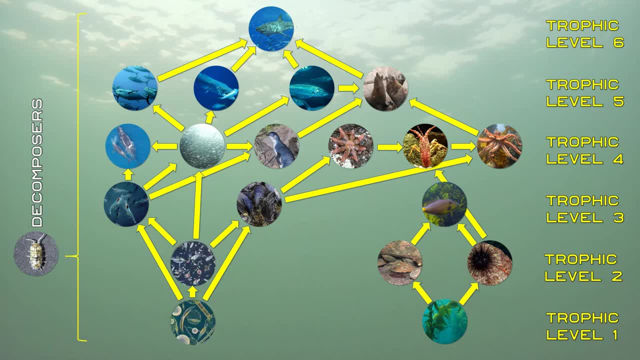 At the lower levels. notice the size of the organisms compared to those higher up the food web. Also think about how many individual organisms exist in the lower levels compared to the number of animals in the higher levels. We can draw a shape over the food web. 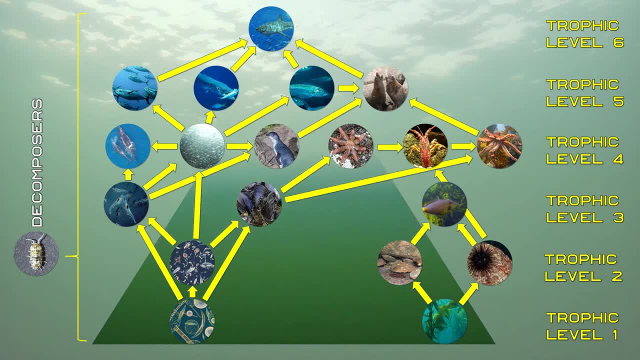 The food web represents the mass of biological matter at each level, and we can see that it forms a triangle with an apex at the top. This is why we call animals at the top of the food chain the apex predators. Here's another thing to think about. What would happen if the conditions in the sea changed to cause a sudden loss of primary producers, such as plankton and algae? The primary consumers wouldn't have anything to eat, so they would die, So then the secondary consumers wouldn't have anything to eat. So they would die, and so on up the food chain. The system would collapse. It can go the other way as well. Removing too many animals from the top of the food chain can have surprising results down the food web. This collapse is called trophic cascade. 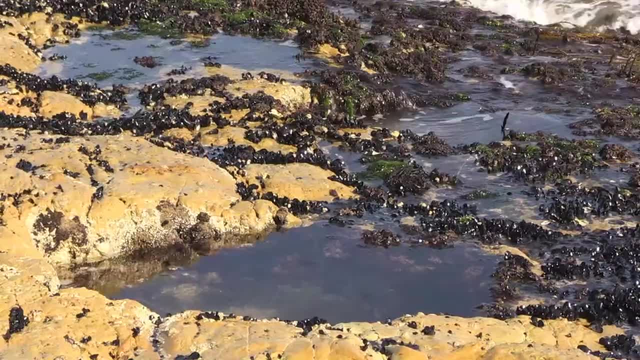 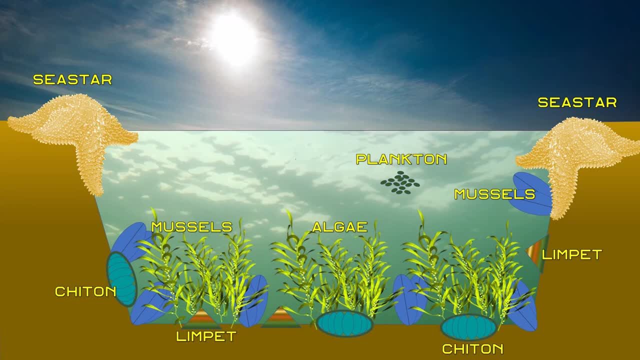 Trophic cascade was discovered by a marine biologist studying rock pools. The food web in the rock pool he was studying looked something like this: The sea stars were the apex predator, and they ate the chitons, limpets and mussels. 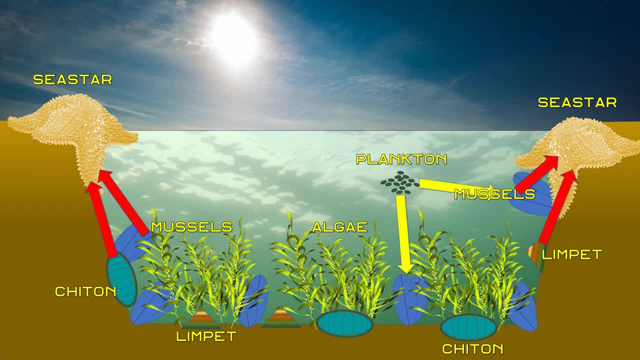 The mussels ate plankton, which were replaced twice a day by the high tide. The chitons and limpets ate the algae. In his experiment, he removed sea stars from some of the rock pools, while leaving other rock pools untouched. as a comparison, 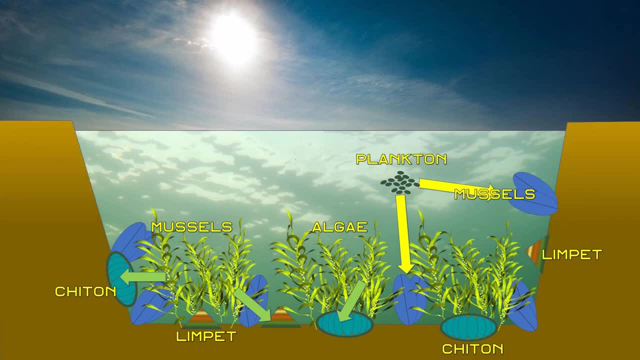 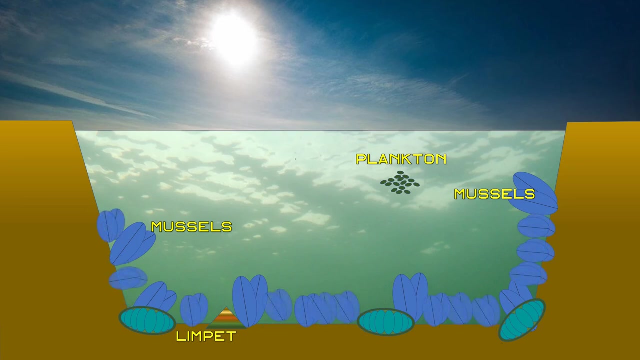 He found that in the pools where the apex predator was removed there was nothing to eat the chitons or limpets, So their populations increased in number, and then they ate most of the algae. The mussels were not being eaten either, and their offspring were able to settle onto the rock where the algae once grew. 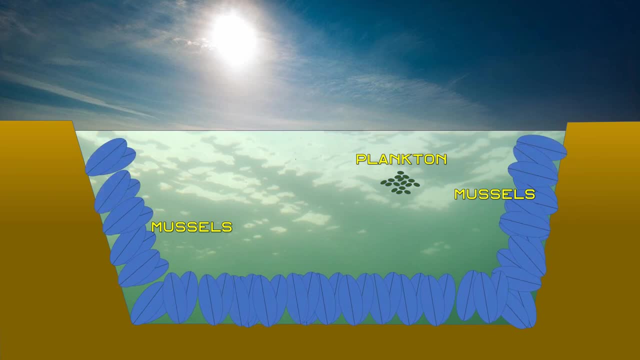 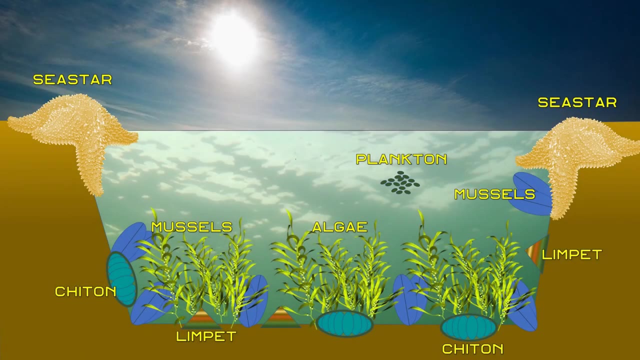 After some time, the rock pools where the sea stars had been removed were covered in mussels, leaving no room or food for limpets or chitons. The flow-on effect of removing an apex predator from the rock pool resulted in an ecosystem with far fewer species.